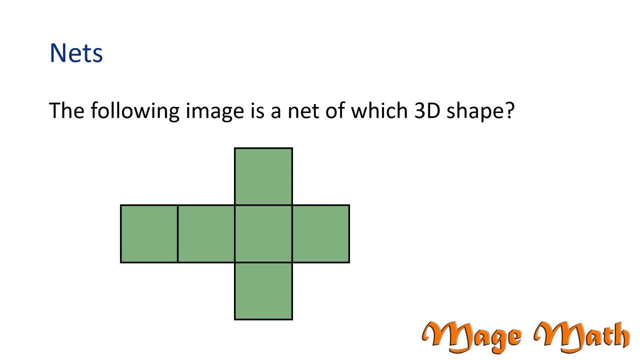 The following image is a model of a solid shape. The following image is a model of a solid shape. The following image is a net of which 3D shape. The figure is comprised of what looks like squares and there are six of them. If we fold along these marked lines, the net will. 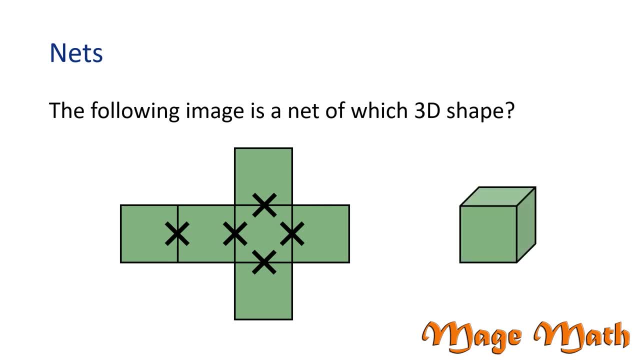 fold into a cube. This is just one net of a cube. There are several more. Can you find another? Let's try this problem. The following image is a net of which 3D shape. This net is made up of two hexagons, which is a type of polygon. 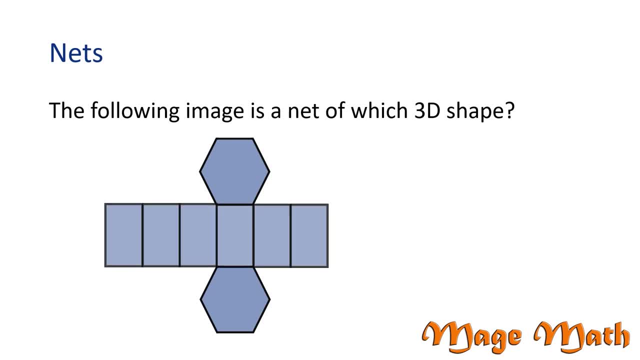 that has six sides and the net also has six rectangles. If we fold along these marked lines, the figure will fold into a type of a prism. Do you know? all prisms have rectangular sides And the specific name of a prism is determined. 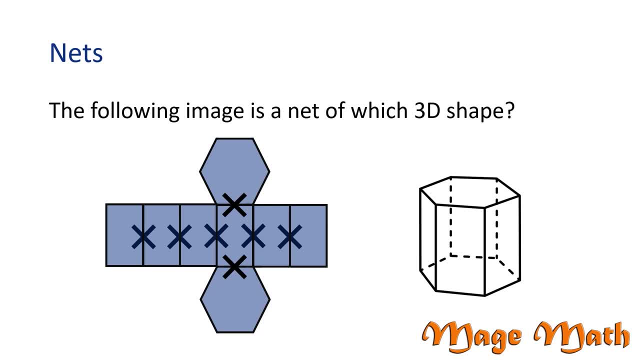 the base shape. Our prism is called a hexagonal prism because the shape of the two bases are hexagons. What about this problem? The following image is a net of which 3D shape. This net is made up of four triangles and one rectangle. If we fold along these marked lines, the figure will 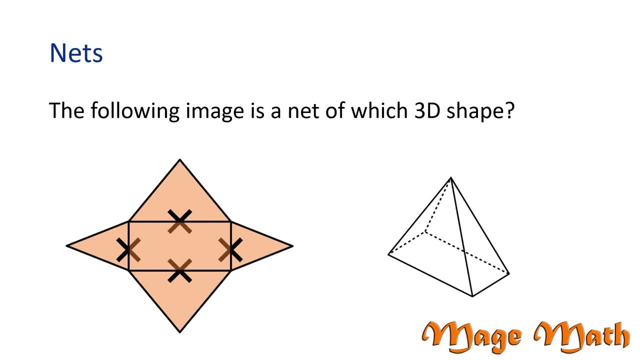 fold into a type of a pyramid. Did you know that all pyramids have triangular sides? The specific name of a pyramid is determined by the base shape. In this case, the base shape is a rectangle, So that's why our net turned into a rectangular-based pyramid. 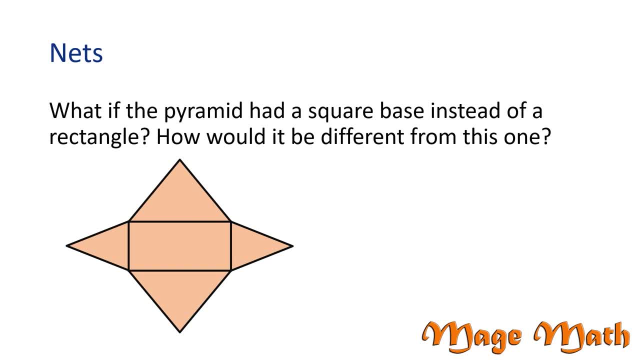 What if the pyramid had a square base instead of a rectangle? How would it be different from this one? What would that net look like? That's right, The base is a square, so the triangles would all be the same size. Hey guys, the bull had lots of fun and wants me to keep riding, but I am taking a break. 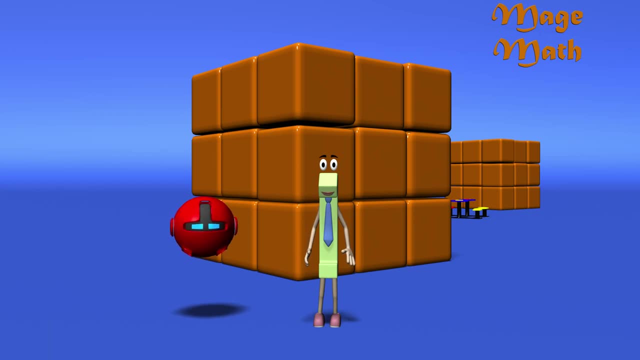 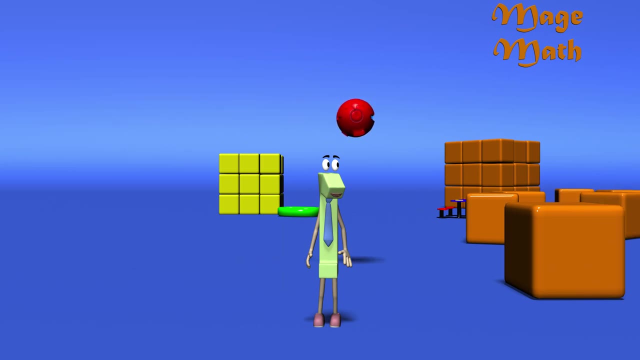 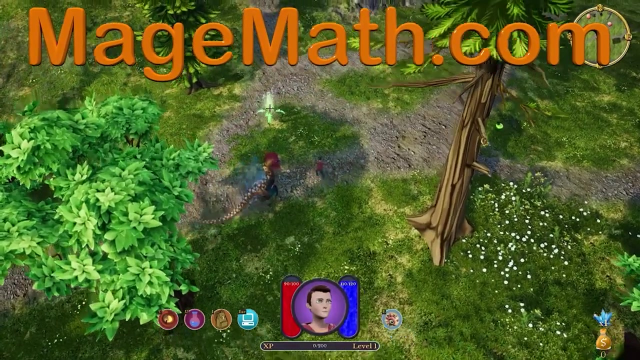 Thanks for learning about nets. Seeing how things fold and move makes 3D really fun. Uh-oh, looks like he wants to play still. See you guys next time. Thank you for watching To support us in making more videos. please check out our game at MageMathcom.